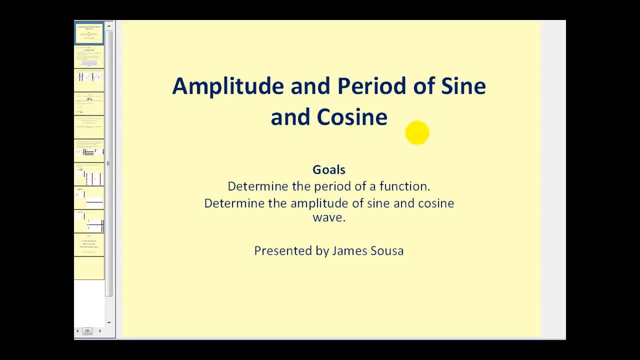 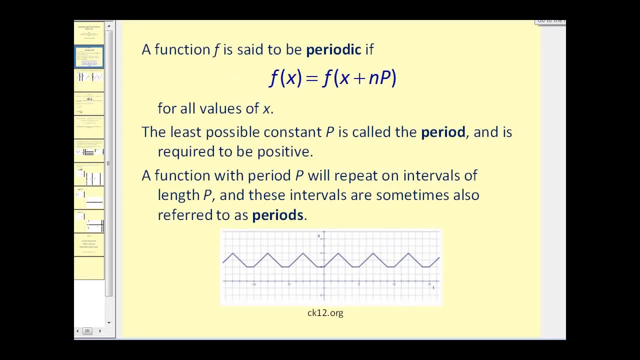 So the goals of this video are to determine the period of a function and then also to determine the amplitude of the sine and cosine wave. A function, f, is said to be periodic if f of x is equal to f of x plus n, p for all values of x, So if these two functions are 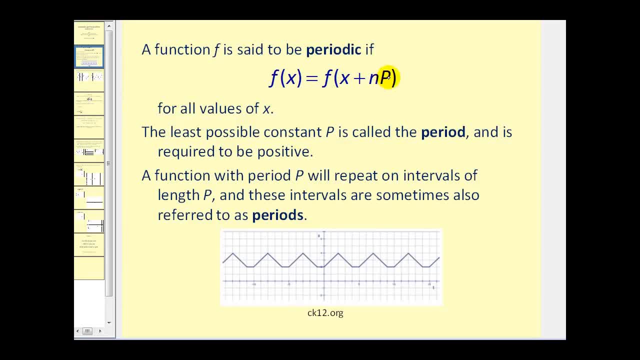 equal, then the least possible constant p is called the period, And the period is required to be positive. A function with period p will repeat on intervals of length p. So if you take a look at this function here, if we start here, when x is equal to zero, 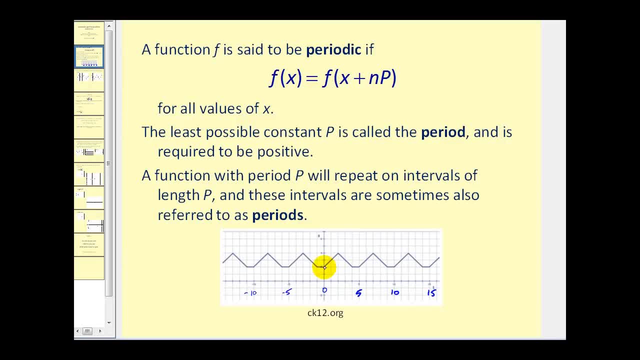 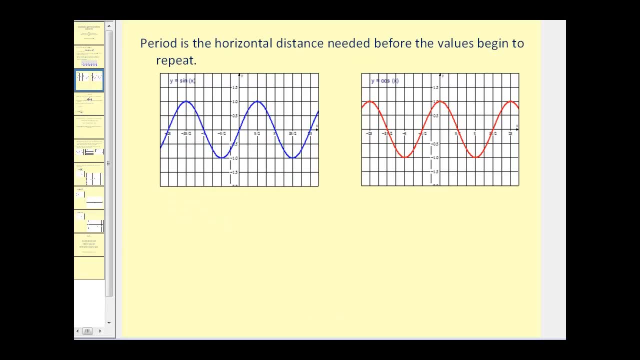 and then we go over to x equals five. this is one complete cycle of the function, because after five it starts to repeat itself Again. the period is the horizontal distance needed before the values begin to repeat. So if we look at the basic sine function, 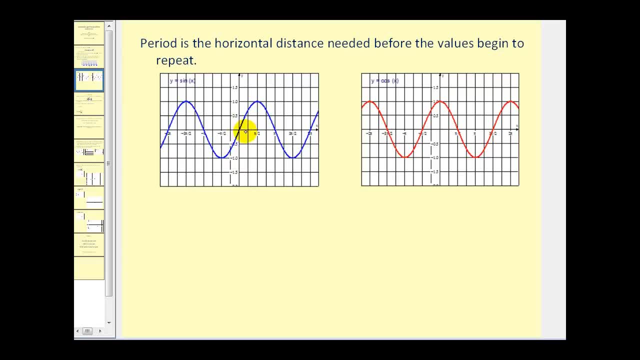 we can see that after the horizontal distance two pi, the function starts to repeat itself. Therefore, the period is equal to two pi for sine theta. And if we take a look at cosine theta, the same thing occurs. After a horizontal distance of two pi, the function would start to repeat itself again. 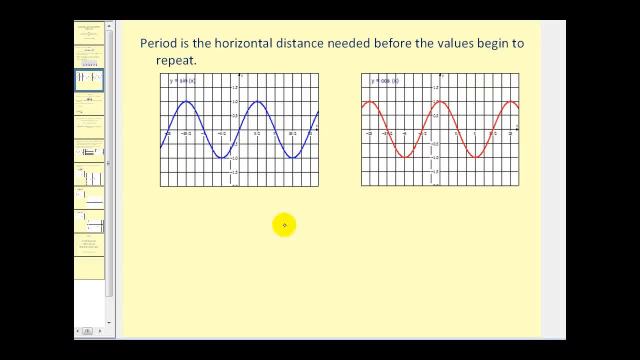 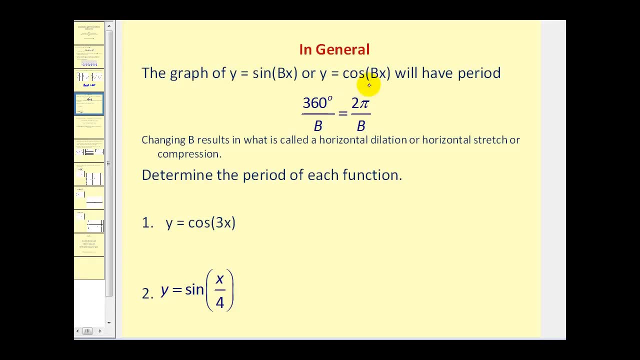 So the period of the basic sine and cosine function is equal to two pi. However, if we take a look at the graphs of y equals sine of bx or y equals cosine bx, the period will change based upon the value of b And in fact the period will be either three hundred sixty degrees divided by b. 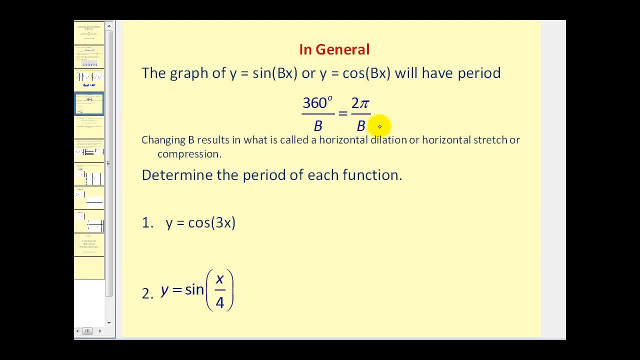 or two pi divided by b, based upon whether we're graphing in degrees Or radians. Changing b results in what is called a horizontal dilation, which can also be called a horizontal stretch or compression. So if we want to determine the period of y equals cosine three x. 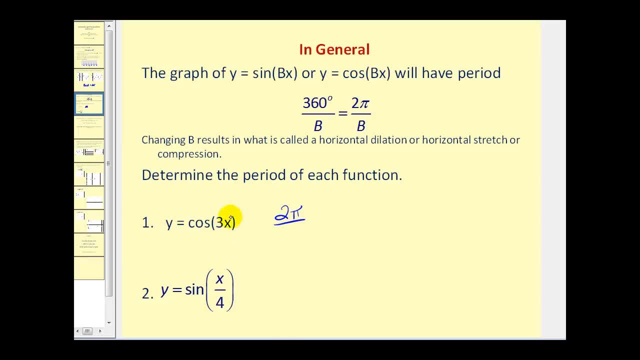 in radians, we would take two pi and divide by the value of b, which is three. This is our period in radians. If we wanted it in degrees, we could take three hundred sixty degrees, divide by three, which is one hundred sixty degrees. 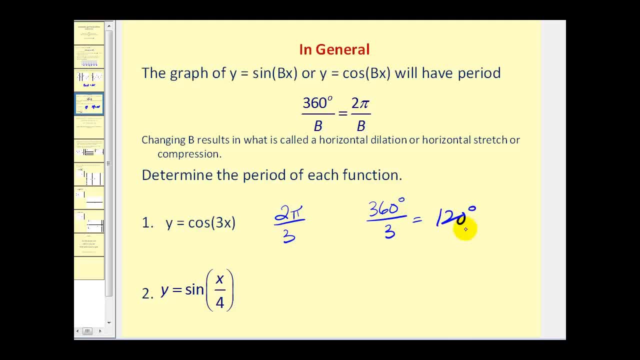 and of course, three pi radians is equal to one hundred twenty degrees. For y equals sine x divided by four. you might want to think of this as one x over four, So the value of b is actually one fourth. Two pi divided by one fourth, remember, is the same as two pi. 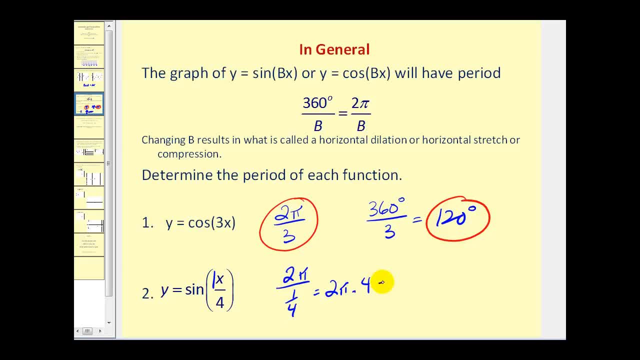 times the reciprocal, So times four over one, or just four, which is equal to eight pi, And this is equivalent to one thousand four hundred forty degrees, And this is equivalent to one thousand four hundred forty degrees, And this is equivalent to one thousand four hundred forty degrees. 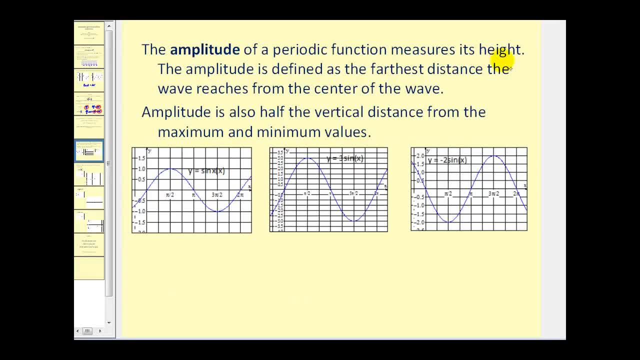 The amplitude of a periodic function measures its height. The amplitude is defined as the farthest distance the wave reaches from the center of the wave. You can also think of the amplitude as half the vertical distance from the maximum and minimum values. So let's take a look at a couple of graphs here. 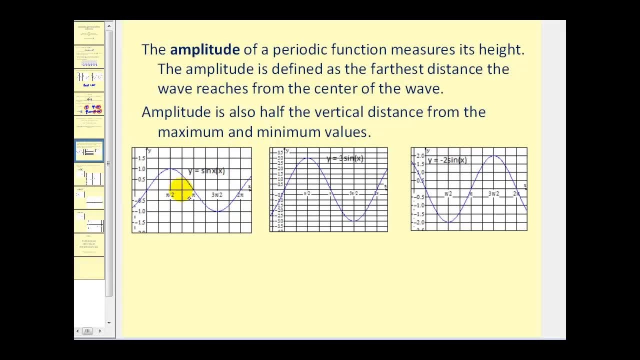 Here we see the graph of y equals sine x. This is the center of the wave and you can see from the center to this maximum is equal to one unit. There's no difference between the center and the maximum. Therefore the amplitude is equal to one. 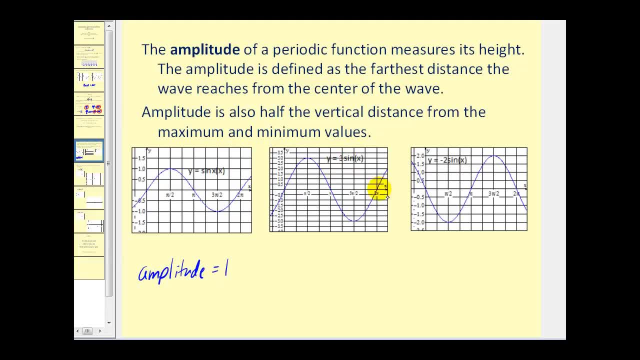 But if you look at the next graph, y equals three sine x. Take a look at the center of the wave again: From the center to the maximum is three units, as well as from the center to the minimum. So the amplitude is now three. 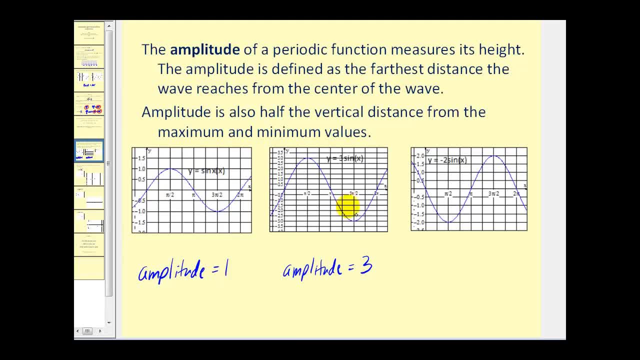 Again, you can think of the amplitude as half the distance from the max to the min. The distance from negative three to three is six units. Half of six, of course, is three. And lastly we have: y equals negative two sine x. 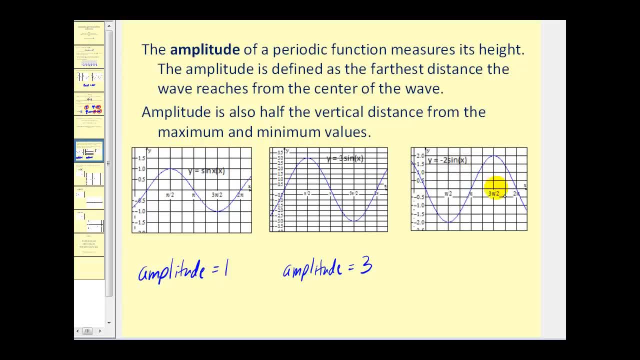 Again, the distance from the center to the max or the min is equal to two units. here, Therefore, the amplitude is equal to two And amplitude always has to be positive. so we do not want to include this negative here. Remember, this negative has the effect of a reflection across the x-axis. 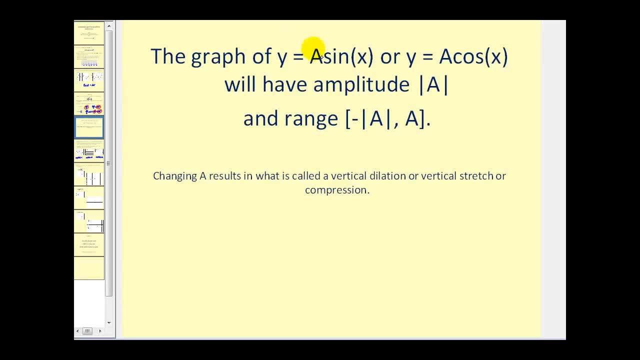 Okay. so in general, if we have the graph of y equals a sine x or y equals a cosine x, the amplitude is the absolute value of a- Remember it always has to be positive- And the range of the amplitude is the absolute value of a. 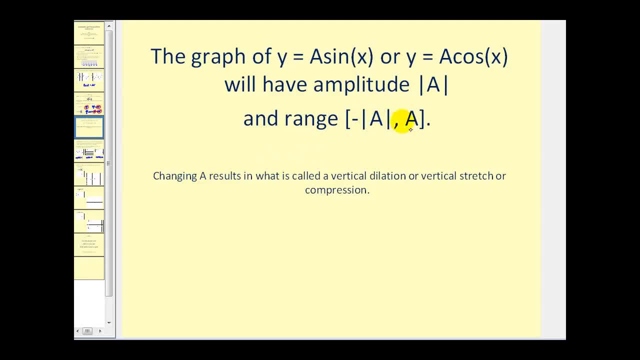 Remember it always has to be positive And the range of the function will be from negative absolute value of a to a on the closed interval. Changing a results in what is called a vertical dilation, which can also be thought of as a vertical stretch or compression. 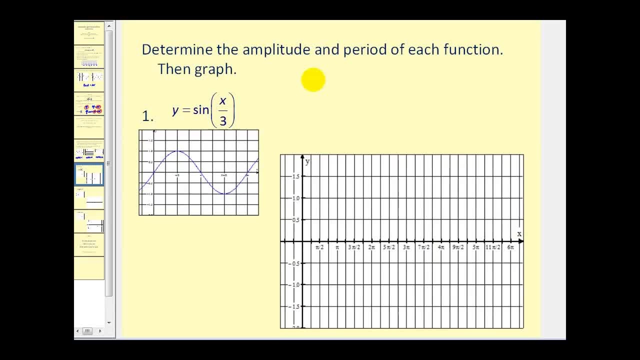 Okay, let's put both of these ideas together by stating the amplitude period and then graphing the function. So we have y equals sine of x divided by three. So from this we can gather that a is equal to one And b would be equal. to remember, there's a one here, so one-third. 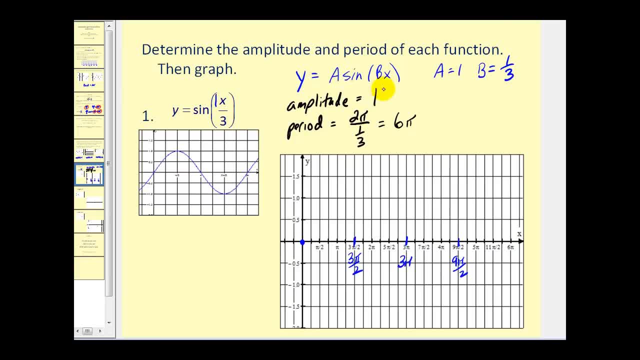 Since a is equal to one or amplitude is equal to one, the period is two pi divided by b. Since b is one-third, two pi divided by one-third is the same as two pi times three over one or six pi. So the next step is we mark off one period on our graph, on our x-axis, from zero to six pi. 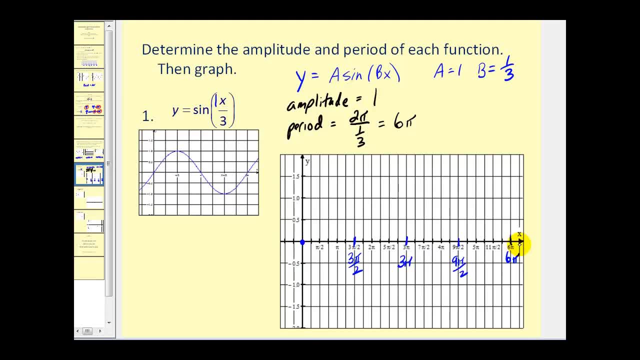 Then we'll divide this interval into four equal parts. So half of six pi would be three pi, and then, dividing it in half again, we'd have three pi over two, And then here we would have nine pi over two. Now, before we begin, let's review the basic sine function here. 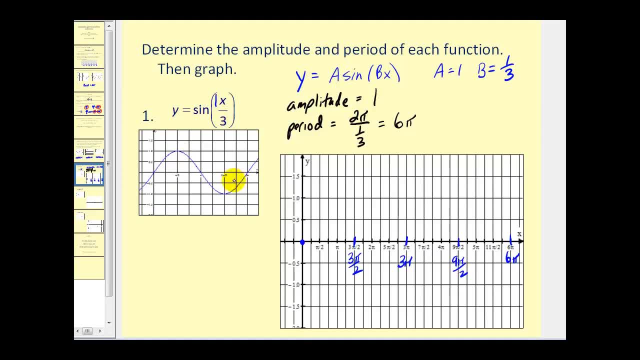 This also has an amplitude of one, but the period has changed for the given function. But that's really the only difference. Notice if we were to take this function and divide it into fourths. Notice if we were to take this period and divide it into fourths. 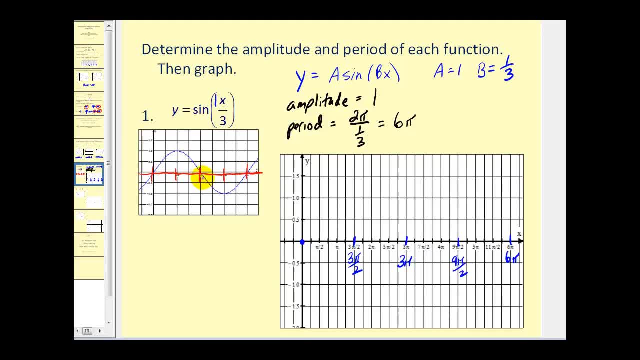 The first fourth would be one-third. That would be our maximum. The second fourth would be back to zero, The third fourth would be at negative one And the fourth fourth would be back at zero for one complete cycle of the sine function. 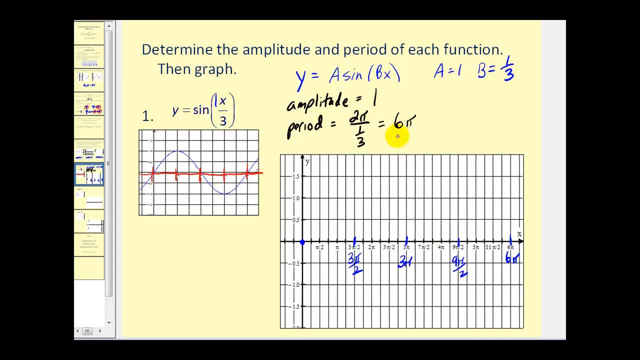 So the only difference here is now our period is six pi, So we're going to start at zero, Then at three pi, over two, we'll be up at one, since our amplitude is still one. At three pi we'll be back at zero. 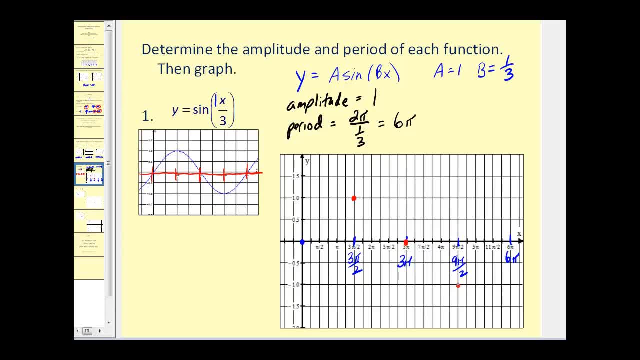 Nine pi over two, we'll be down at negative one, And then at six pi we'll be back at one. And now we can make a nice graph of y equals sine of x divided by three. Notice the graphs look very similar. 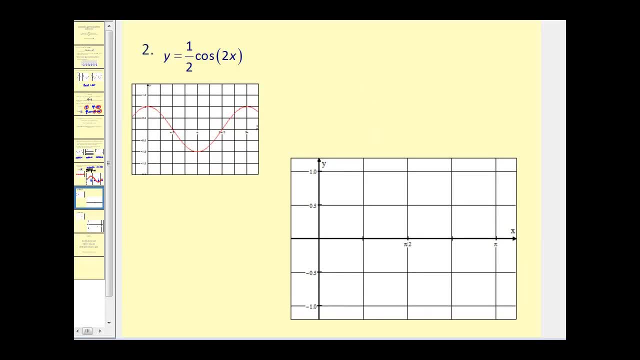 The only difference is we have a different period. Now let's graph y equals one-half cosine two x. Notice: for reference we'll use the basic graph of y equals cosine theta. Okay, so from this we can gather that a is equal to one-half. 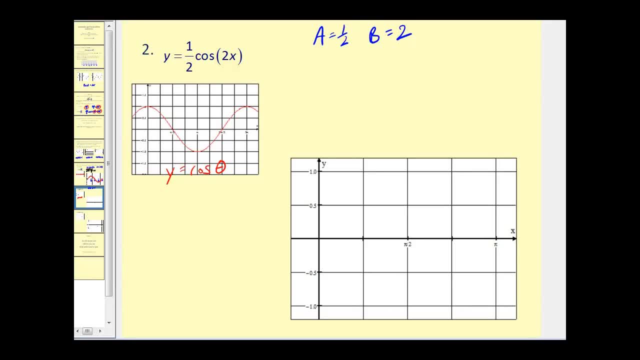 And b is equal to two. Since a is one-half, our amplitude is equal to one-half And our period is equal to two pi divided by b. So we have a period of pi radians. First step would be to mark off pi radians on the x-axis. 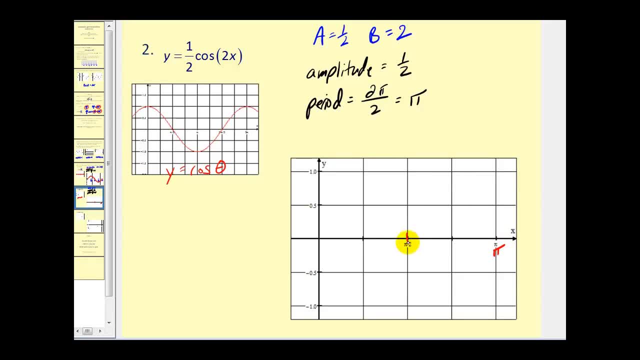 Divide it into four equal parts. So here's our pi. Then we have pi over two. This would be pi over four, And this would be three pi over four. Again, notice that for zero radians the basic cosine function is equal to positive one. 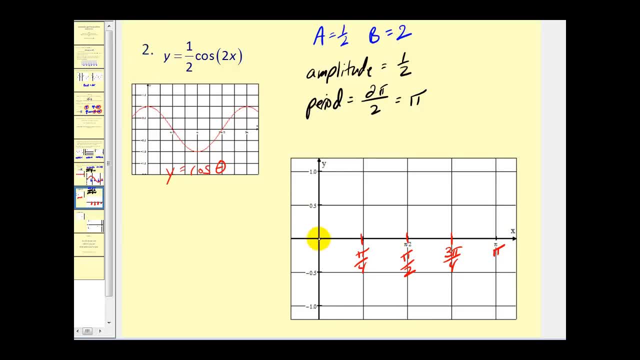 Well, if our amplitude is now only one-half at zero radians, the function value will be one-half rather than one. And now the pattern will be consistent: At the next fourth we'll be down at zero. At the next fourth we'll be down at negative one. 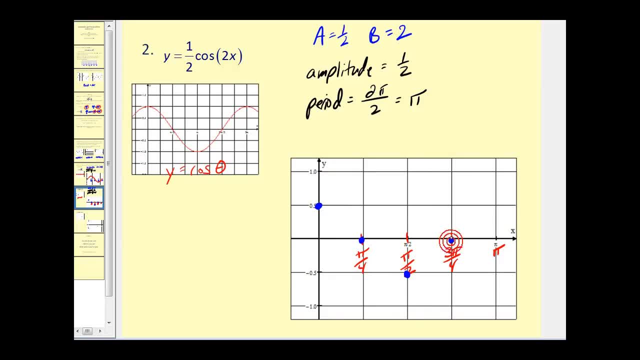 But in this case negative: one-half Back to zero And then back up to one-half. These points are enough to make a nice graph of y equals one-half cosine two x. Now notice that these functions look almost the same, But what we've changed is how we scaled the x-axis. 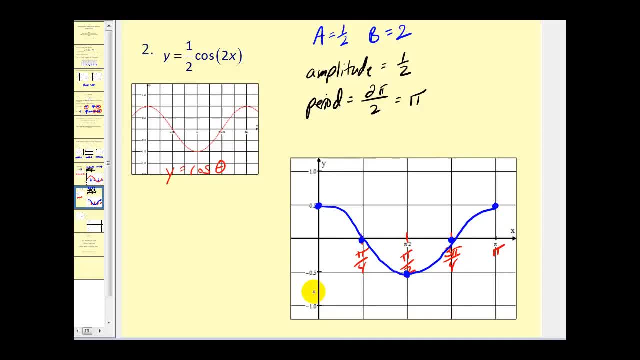 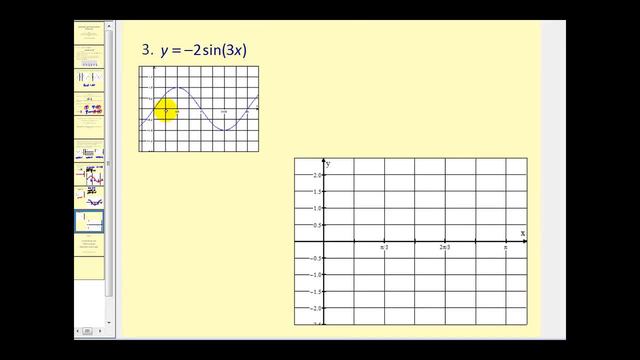 and how we scaled the y-axis. Let's go ahead and try one more. Now. we have y equals negative two sine three x. Notice again for reference: we have y equals sine theta. This should help us see the pattern for the new graph. 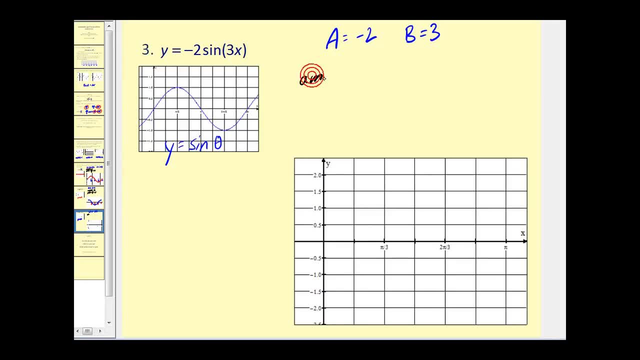 Remember, the amplitude is equal to the absolute value, So it's equal to two. And the period is equal to two pi divided by b. So our period is two pi divided by three. So we'll start by marking off our x-axis at two pi over three. 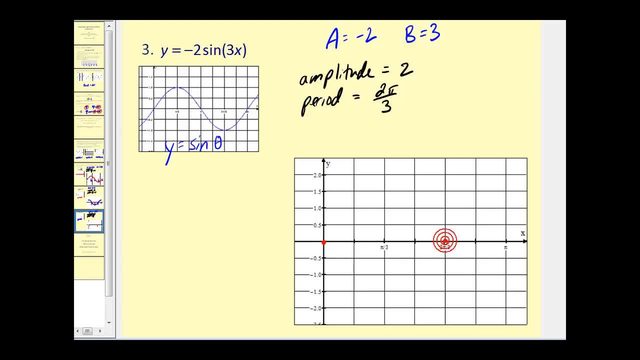 So here we have zero, two pi over three. here We'll divide this interval into four equal parts. So in the middle we have pi over three. Half of that would be pi over six And half the distance between pi over three and two pi over three. 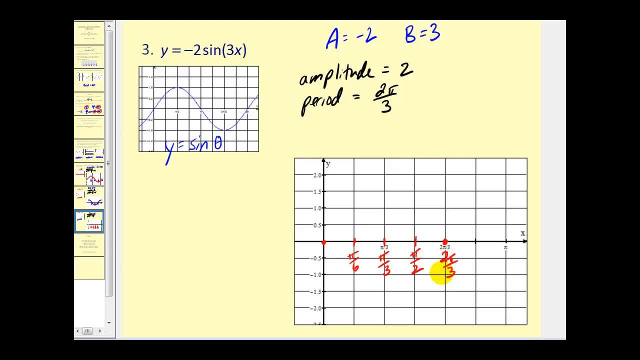 would be pi over two. Okay, remember that at zero radians the basic sine function is equal to zero. So that'll still be true here. But now on the basic sine function, the first, fourth, we're up at positive one, Since the amplitude is two. 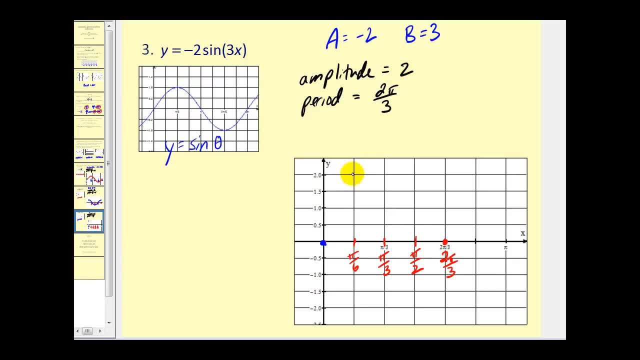 we might think we're going to be up at positive two, But remember that this negative here results in a reflection across the x-axis, So we're actually down at negative two. So you do have to be careful. When a is negative, you do have to reflect.